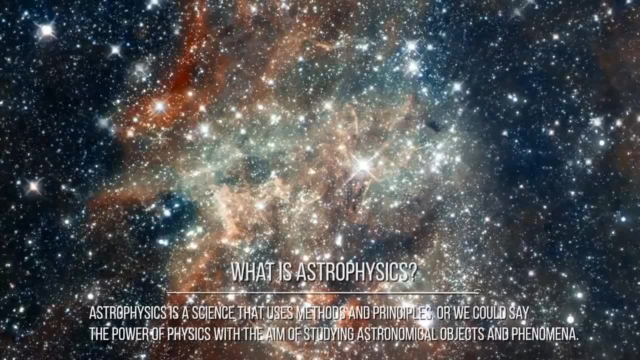 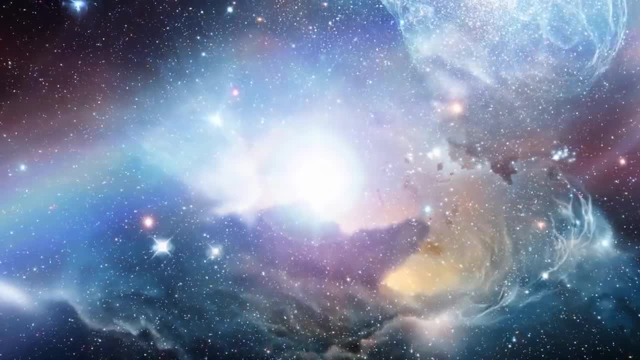 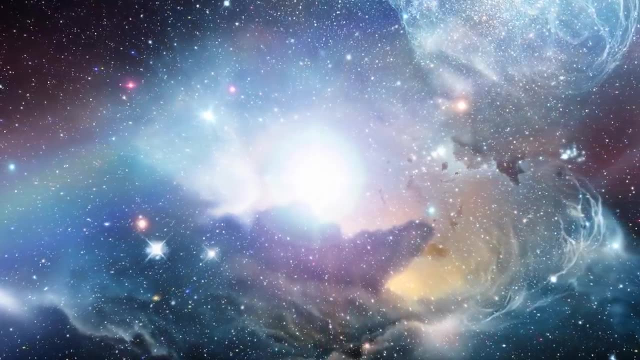 or we could say the power of physics, with the aim of studying astronomical objects and phenomena. Of course, among the subjects studied are the sun, other stars and galaxies, But astrophysics also studies extrasolar planets, the interstellar medium and the cosmic microwave background. How can scientists study these objects? How is 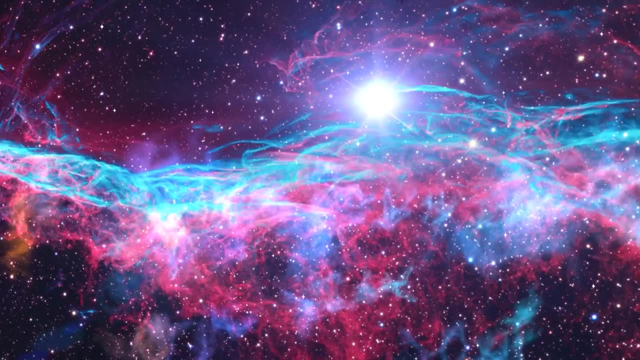 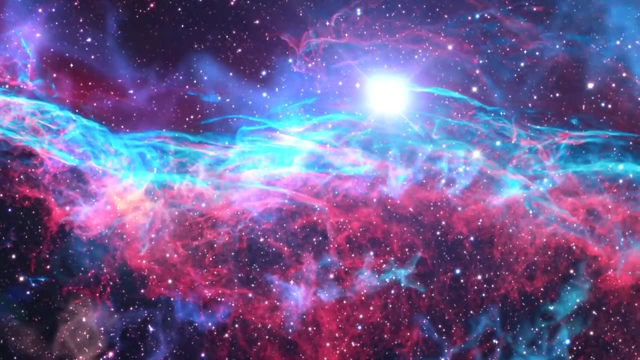 it done Well, they study their emissions. In fact, every object has its own emission, which we can think of as the intrinsic energy of the object that produces a spectrum. Emissions from these objects are examined across all parts of the electromagnetic range and the properties. 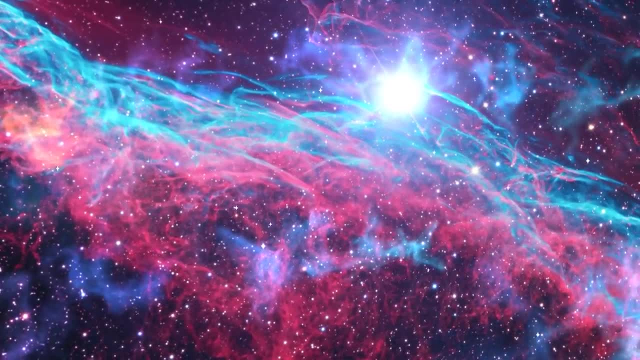 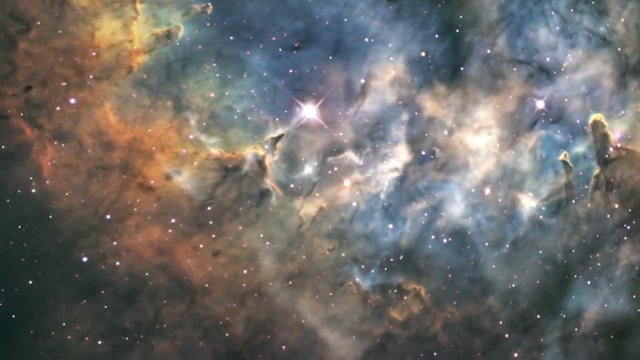 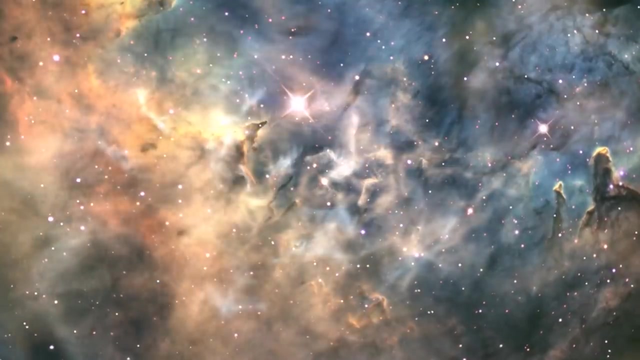 examined include luminosity, density, temperature and chemical composition. Astrophysics is a very broad subject and it applies concepts and methods from many disciplines of physics, including classical mechanics, electromagnetism, statistical mechanics, thermodynamics, quantum mechanics, relativity, nuclear and particle physics and atomic and molecular physics. 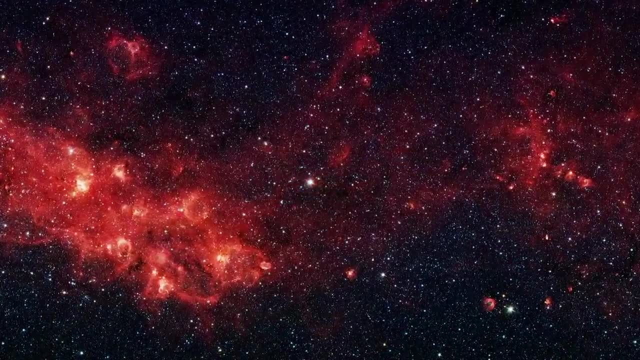 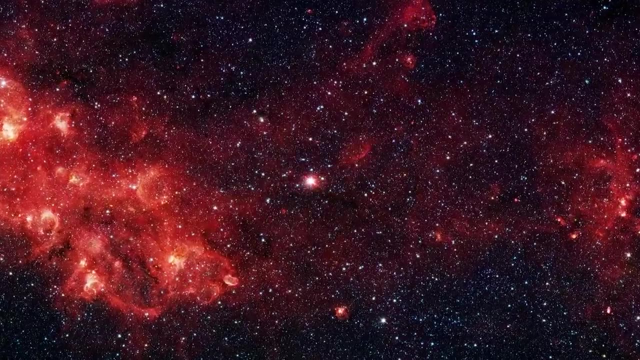 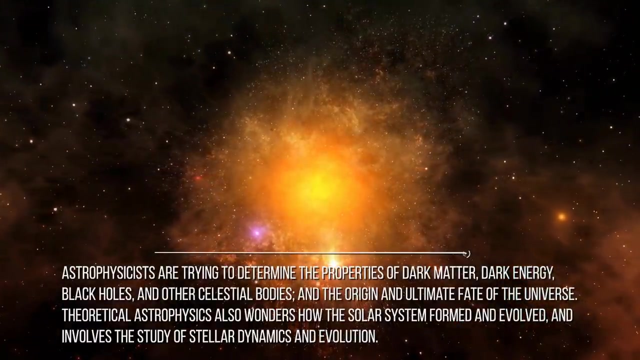 That's why one has to study a lot in order to become an astrophysicist. In practice, modern research often involves a huge amount of work in the realms of both theoretical and observational physics. Astrophysicists are trying to determine the properties of dark matter, dark energy, black holes and other celestial bodies. 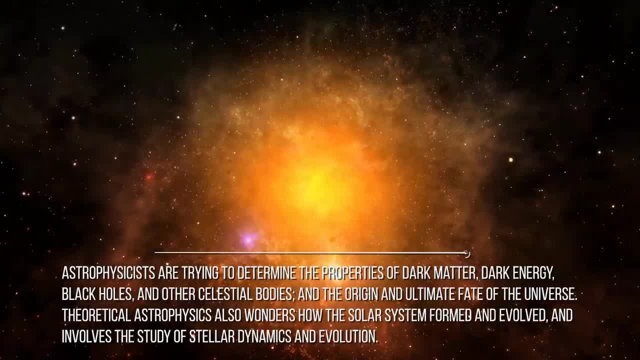 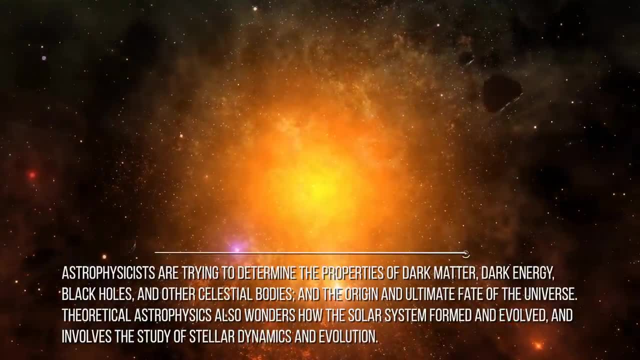 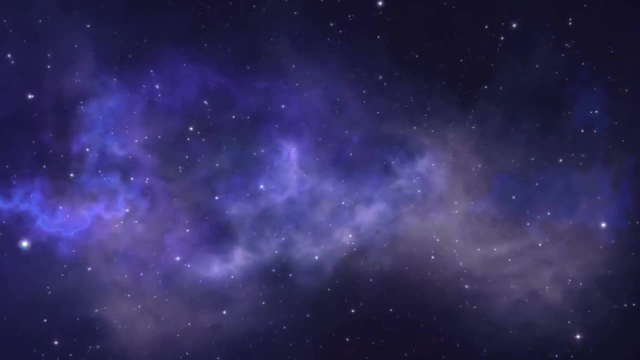 and the origin and ultimate fate of the universe. Theoretical astrophysics also wonders how the solar system formed and evolved, and involves the study of stellar dynamics and evolution. We said that astrophysicists study the spectrum of celestial objects, but what exactly is a spectrum? All normal matter emits electromagnetic. 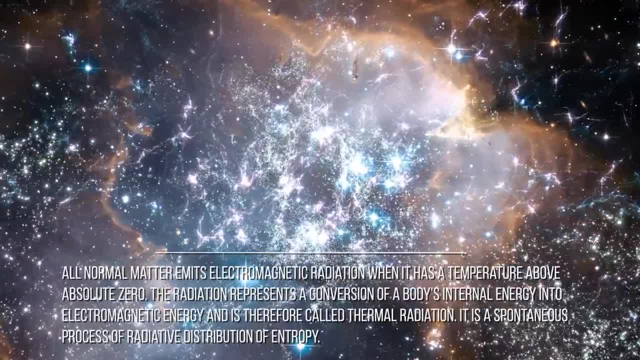 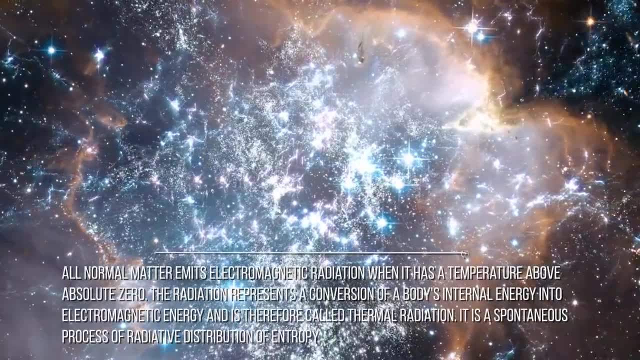 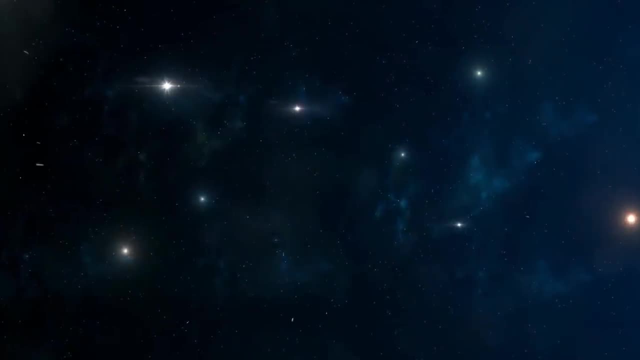 radiation when it has a temperature above absolute zero. The radiation represents a conversion of a body's internal energy into electromagnetic energy and is therefore called thermal radiation. It is a spontaneous process of radiative distribution of entropy. Conversely, all matter is a state of being that absorbs electromagnetic radiation to some degree. 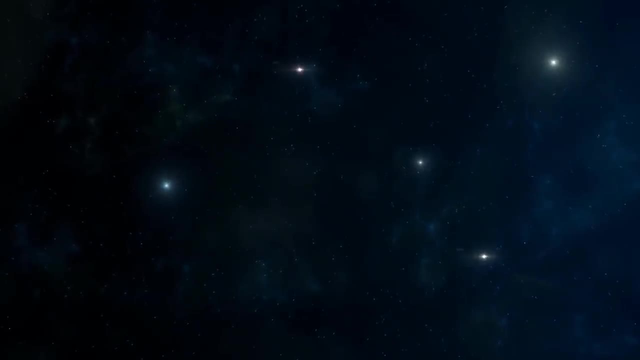 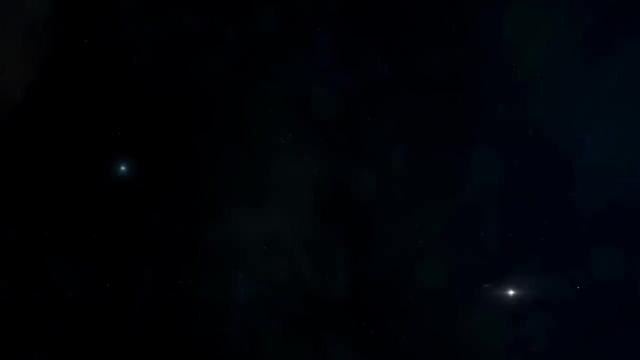 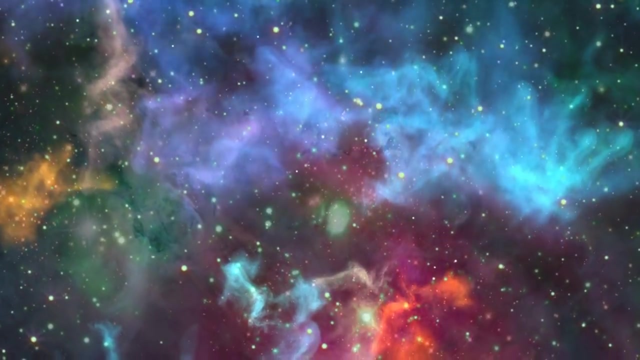 An object that absorbs all radiation falling on it at all wavelengths is called a blackbody. When a blackbody is at a uniform temperature, its emission has a characteristic frequency distribution that depends on the temperature. Its emission is called blackbody radiation. The spectrum of a star is composed mainly of thermal radiation that produces a continuous 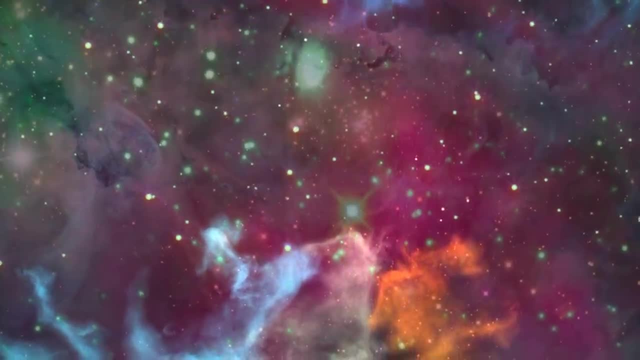 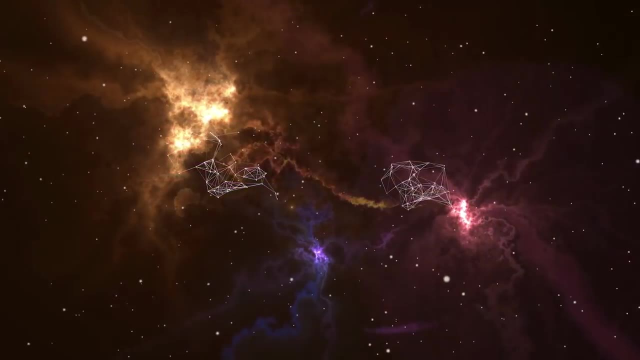 spectrum. The star emits light over the entire electromagnetic spectrum, From gamma rays to radio waves. however, stars do not emit the same amount of energy at all wavelengths. Nowadays, we are well aware of all these things, but at the end of the 19th century 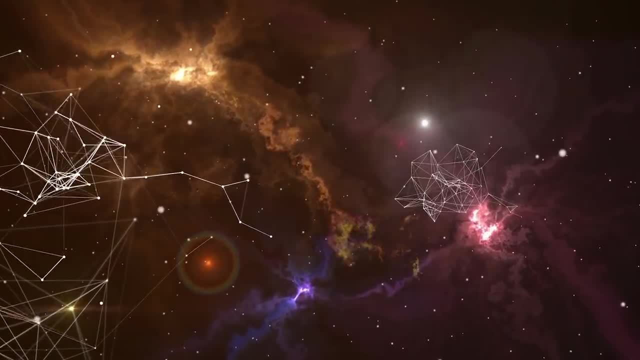 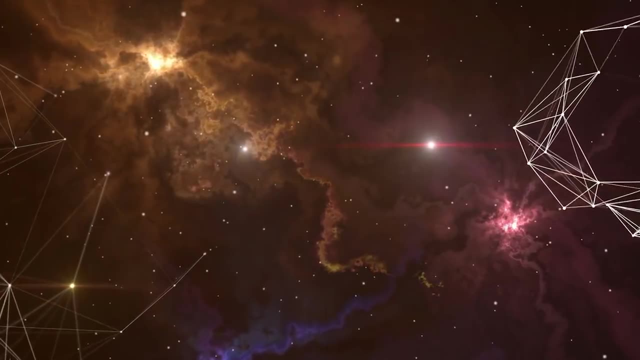 physicists were unable to explain why the observed spectrum of blackbody radiation, which by then had been accurately measured, diverged significantly at higher frequencies from that predicted by existing theories. Blackbody radiation is the thermal electromagnetic radiation. within the solar system, The blackbody radiation is the thermal electromagnetic radiation. 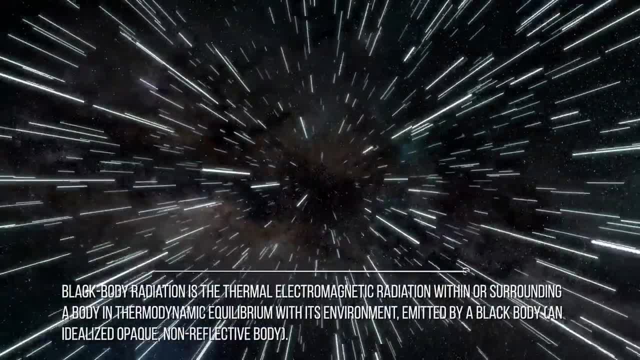 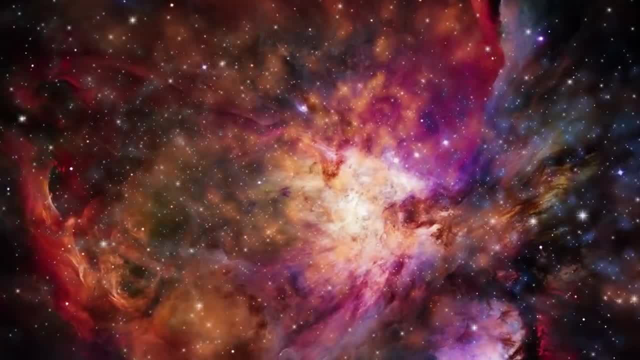 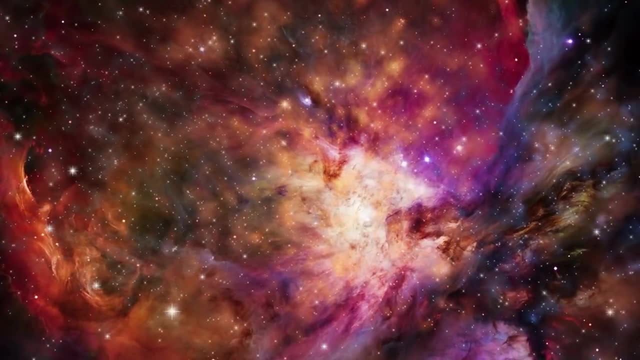 within or surrounding a body in thermodynamic equilibrium with its environment, emitted by a blackbody, an idealized opaque, non-reflective body. The concept of the blackbody is in fact an idealization, as perfect blackbodies do not exist in nature. Graphite and lamp black with 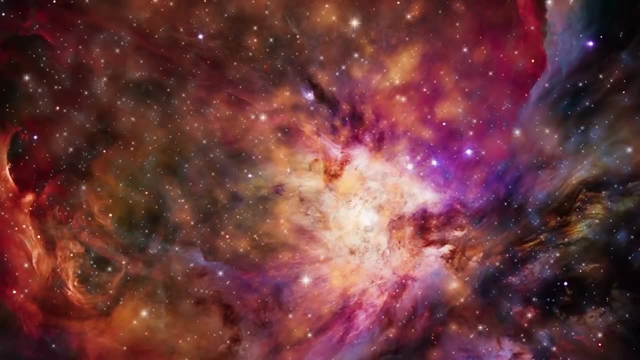 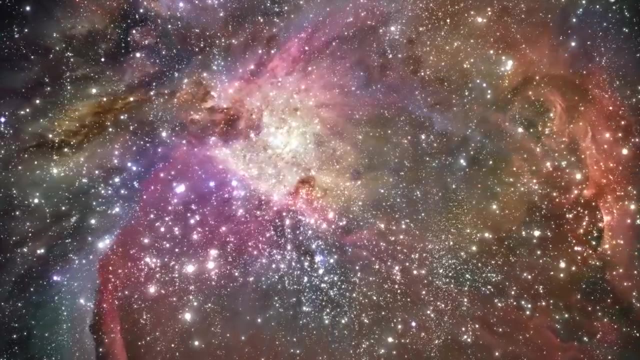 emissivities greater than 0.95,, however, are good approximations to a black material. In 1900, Max Planck derived a formula for the observed spectrum of a blackbody. The Planckian function is a function of only the frequency of the radiation and the body's 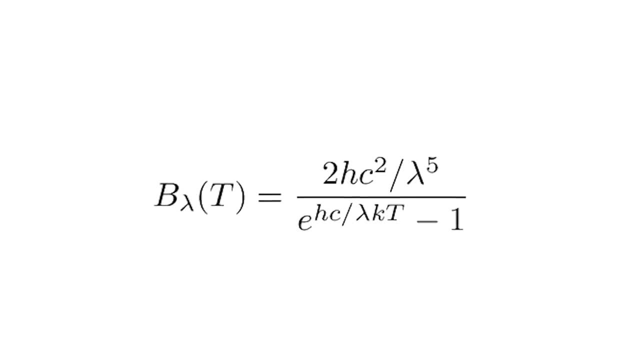 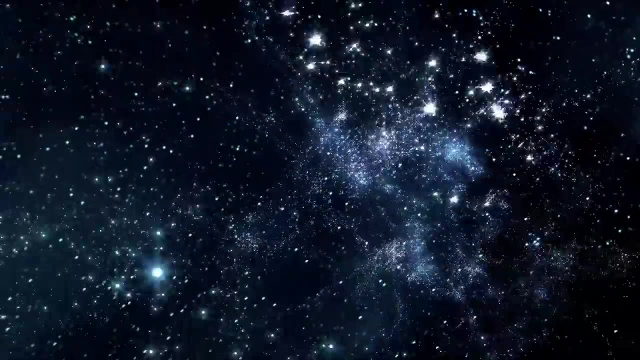 temperature. A typical Planckian function looks like this. Today we know stars can in first approximation be thought of as blackbodies, but their observed spectrum is not an exact Planckian function. This is because, as we stressed before, 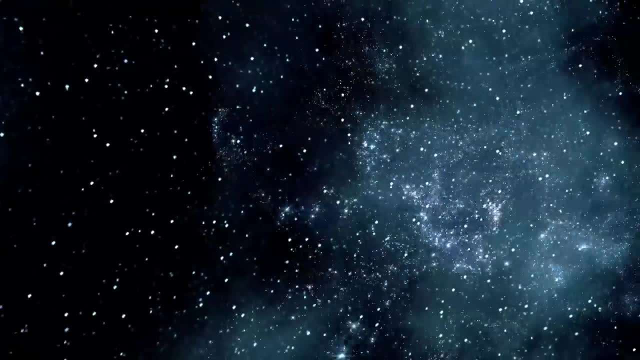 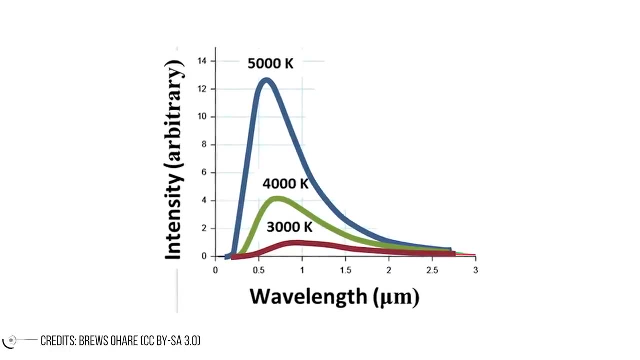 blackbodies are an idealization, something that doesn't really exist in nature. Here's the observed flux for a star. As you can see, it looks pretty different from the Planckian function and it seems there are some lines missing. What caused them? 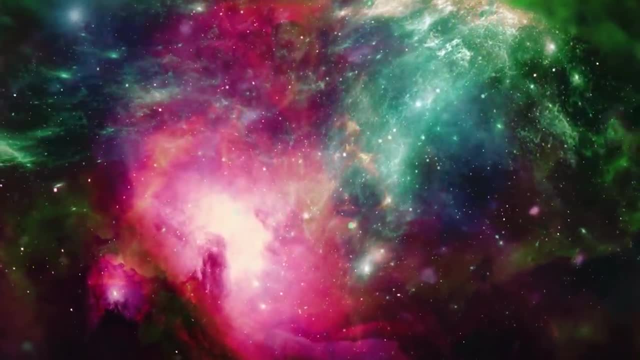 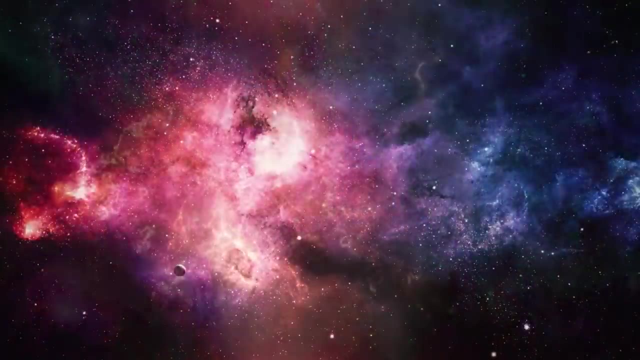 This was a difficult question to answer, but then, at the end of the 19th century, scientists Kirchhoff and Bunsen entered the game and nothing stayed the same. It's time to give a proper answer to our second question: What's spectroscopy? 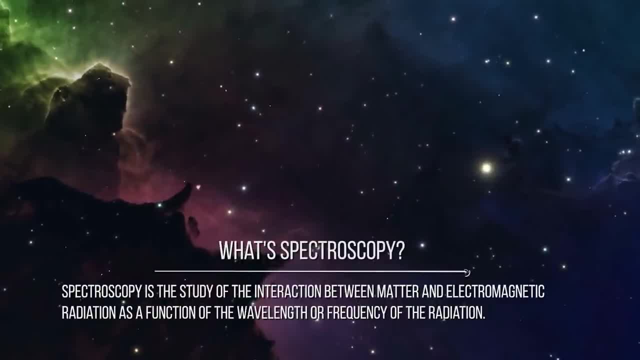 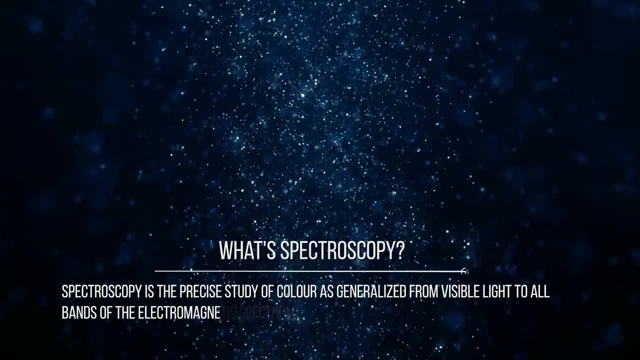 Spectroscopy is the study of the interaction between matter and electromagnetic radiation as a function of the wave's energy. This is the study of the interaction between matter and electromagnetic radiation as a function of the wave's energy. In simple terms, spectroscopy is the precise study of color as generalized. 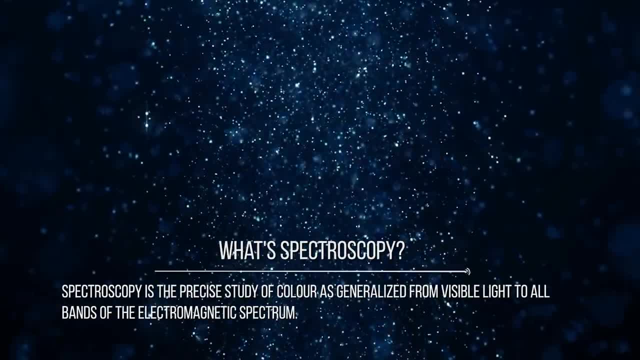 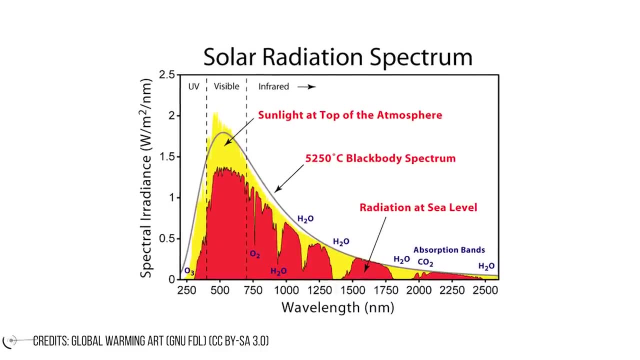 from visible light to all bands of the electromagnetic spectrum. We could say that in 1859, Gustav Kirchhoff and Robert Bunsen gave birth to spectroscopy. Bunsen reported to a colleague that Kirchhoff had made a totally unexpected discovery. 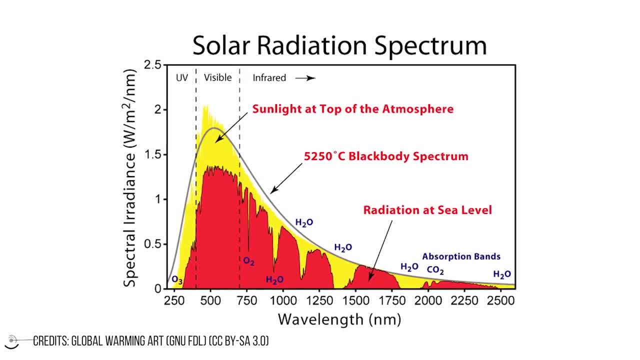 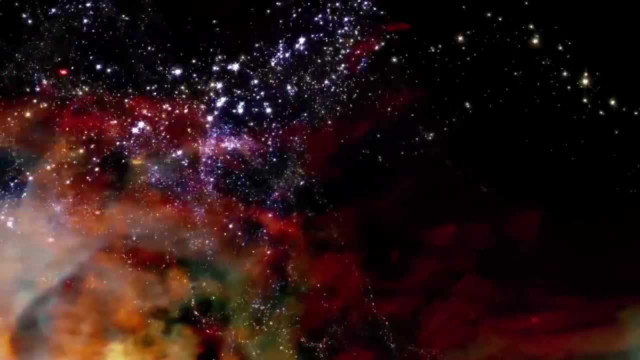 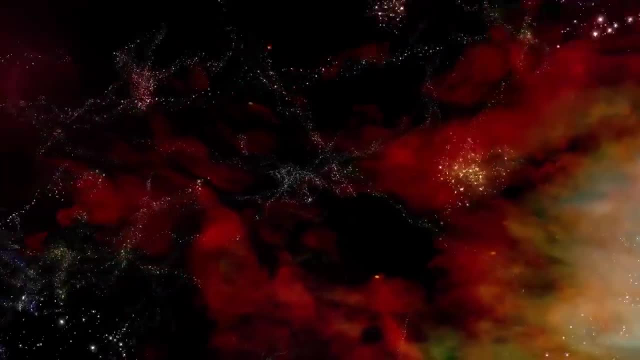 He had identified the cause of the dark lines seen in the solar spectra. When certain chemicals were heated in Bunsen's burner, characteristic bright lines appeared. In some cases these were at exactly the same points in the spectrum as the solar spectrum dark lines. The bright lines were light coming from hot gas. 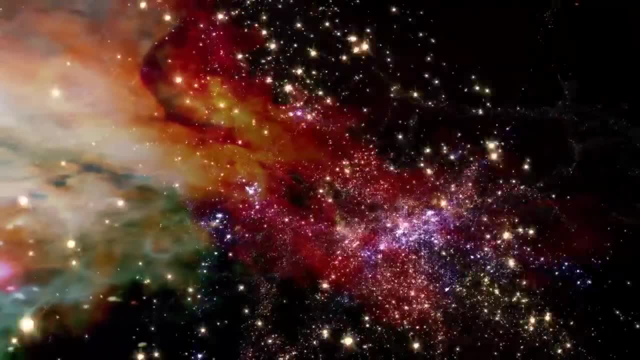 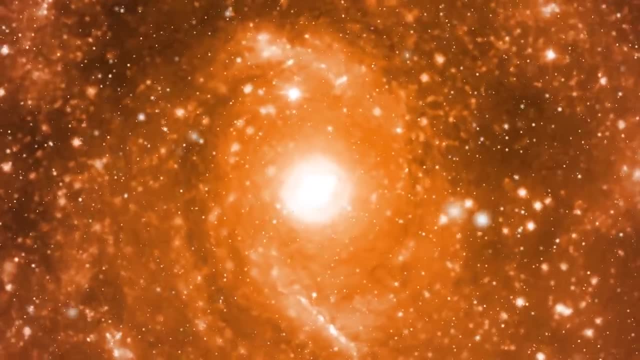 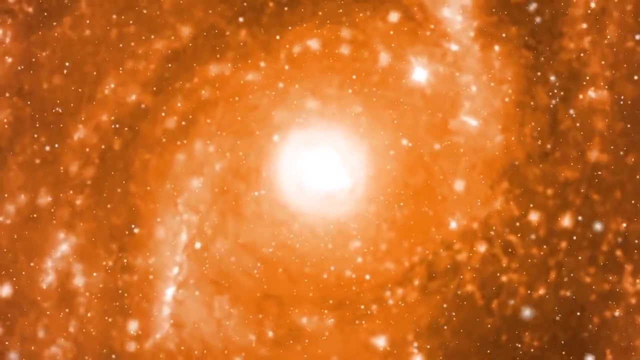 whereas the dark lines showed an absorption of light in the cooler gas above the sun's surface. The two scientists found that every chemical element produces a unique spectrum. This provides a sort of fingerprint which can confirm the presence of that chemical. Kirchhoff and Bunsen recognized that this could be a powerful tool for the determination. 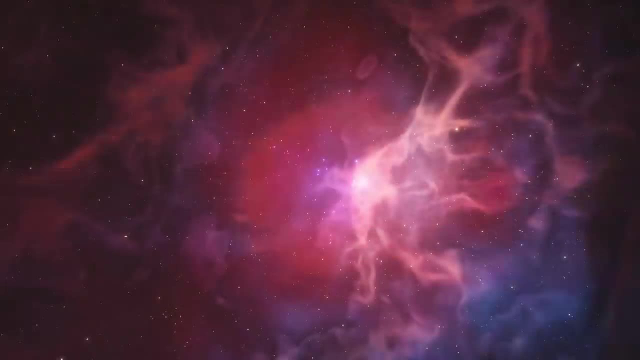 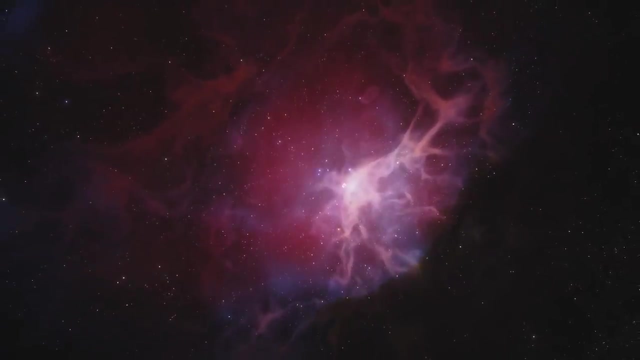 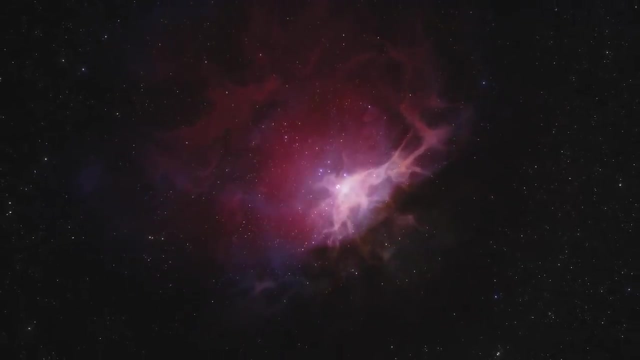 of the chemical composition of the sun and stars. And they were right. Astronomers and astrophysicists couldn't live today without spectroscopic surveys. The types of spectroscopy can be distinguished by the nature of the interaction between the energy and the material. These interactions include: 1. Absorption- spectroscopy, absorption occurs. 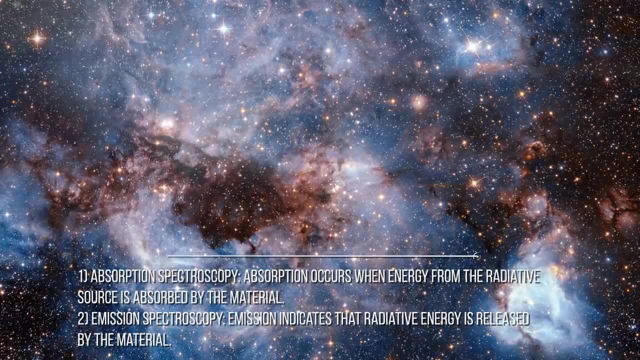 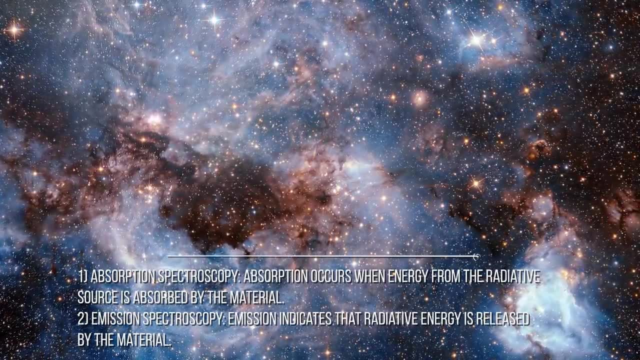 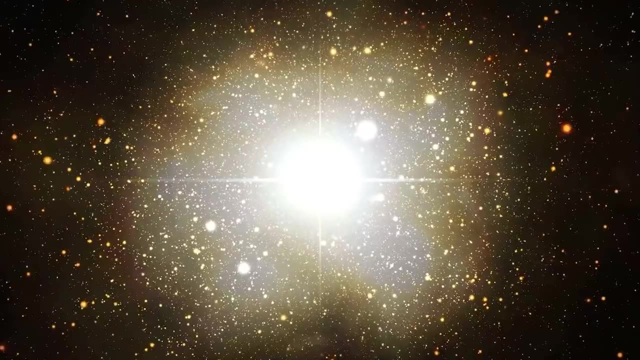 when energy from the radiative source is absorbed by the material. 2. Emission- spectroscopy. Emission indicates that radiative energy is released by the material. Spectroscopy is so important that British astronomer and chemist Warren de la Rue in 1861. 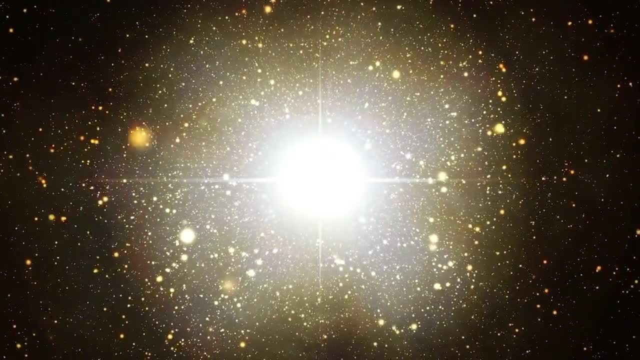 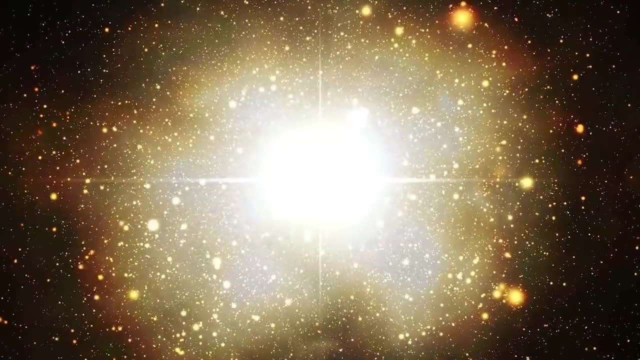 stated, if we were to go to the sun and to bring some portions of it and analyze them in our laboratories, we could not examine them more accurately than we can by this new mode of spectrum analysis. Now that we know what spectroscopy is, we can understand better how. 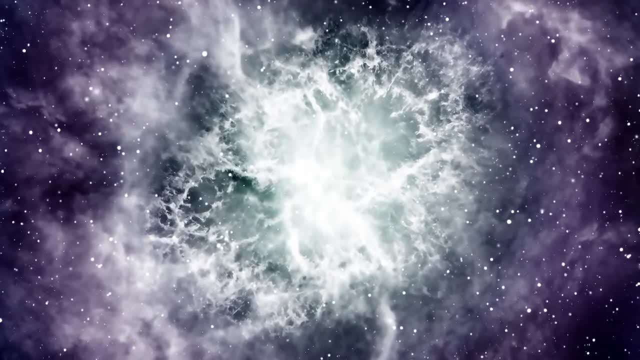 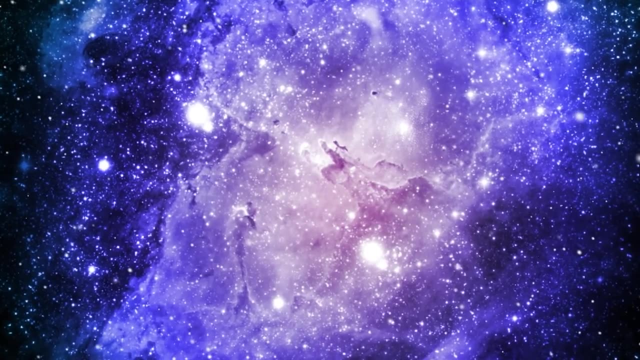 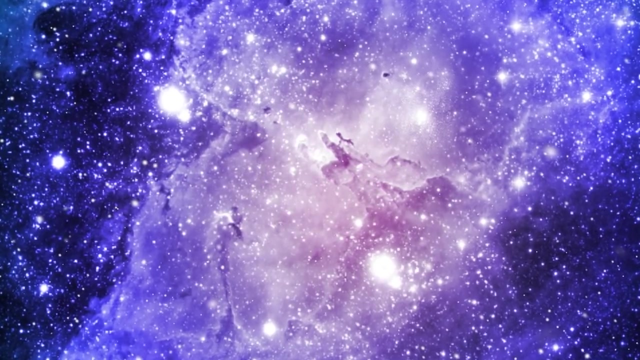 astrophysicists study star positions, masses, velocities and all the other physical features of celestial bodies. In fact, spectroscopy provides us with positions of stars and gas clouds, For example. with the help of spectroscopy, we can understand better the spatial distribution of 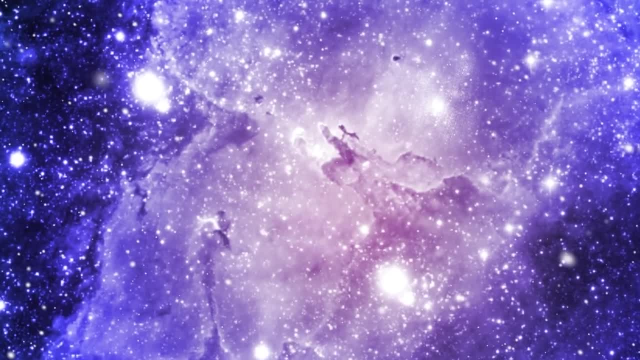 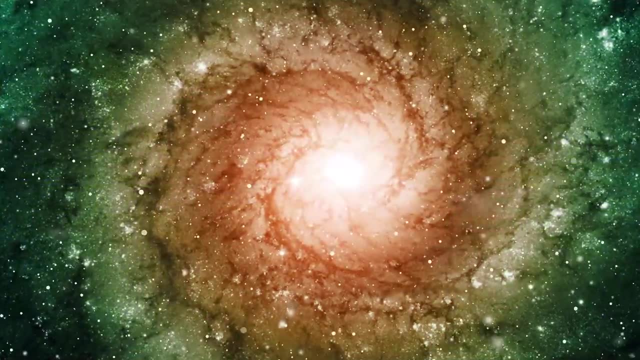 stars in our galaxy. Also, using the so-called Virial theorem, we can infer stellar masses and chemical abundances of elements with respect to hydrogen. And, last but not least, we use spectroscopy to study velocities. How do we? Well, maybe you've already heard. 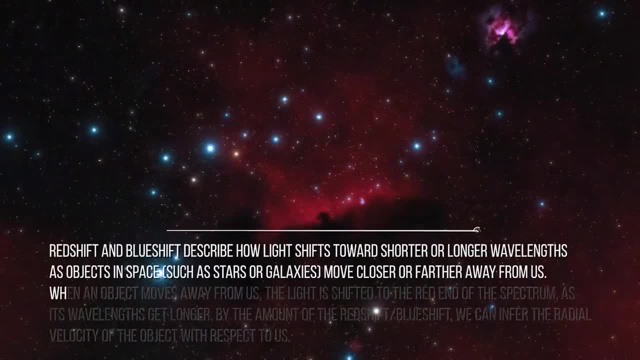 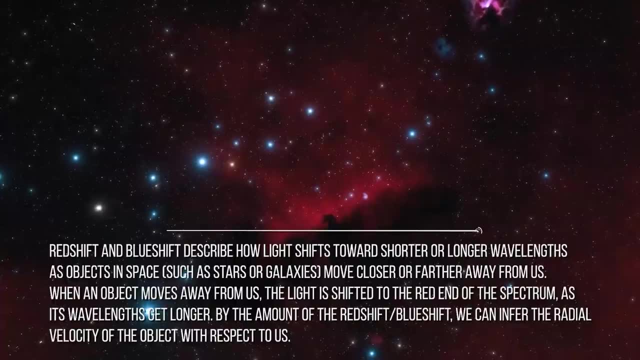 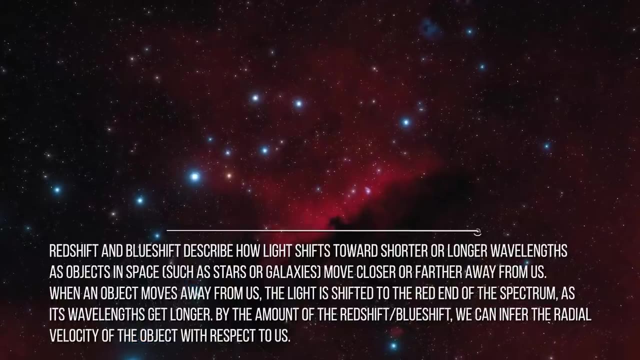 about redshift and blueshift. Redshift and blueshift describe how light shifts towards shorter or longer wavelengths as objects in space, such as stars or galaxies, move closer or farther away from us. When an object moves away from us, the light is shifted to the red end of the spectrum. 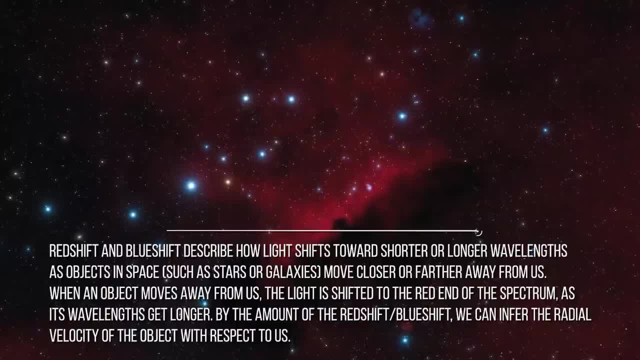 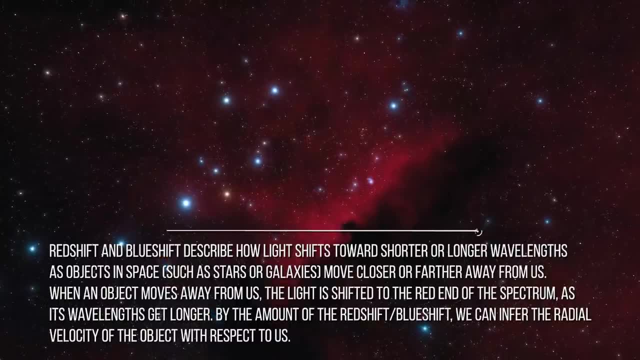 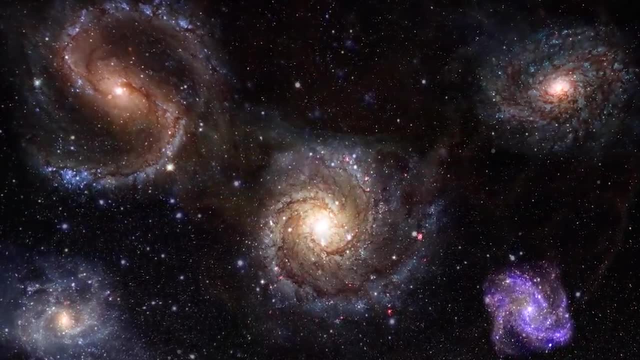 as its wavelengths get longer. By the amount of redshift-blueshift we can infer the radial velocity of the object with respect to us. Isn't it amazing. Studying colors equals studying the universe. What does an astrophysicist do? An astrophysicist may perform research on the planets. 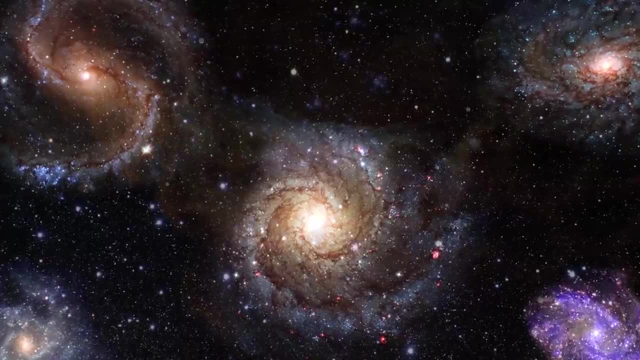 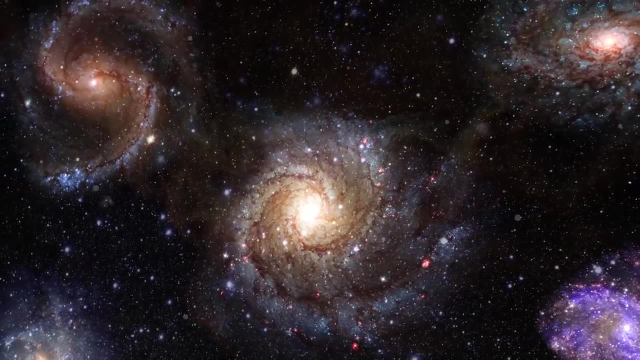 the stars, other galaxies and objects in the universe. They take an in-depth knowledge of physics and apply it to astrological theories. An astrophysicist may have the following responsibilities: Develop astrological theories and implement research techniques to test those theories. 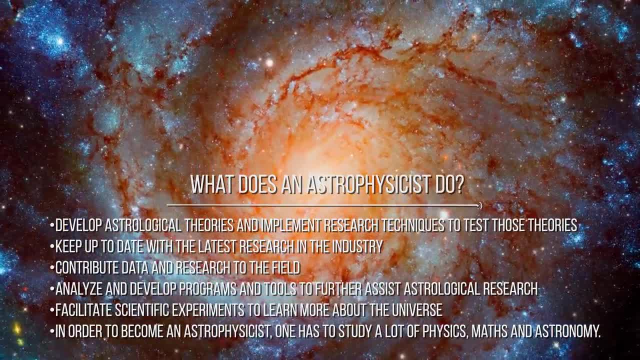 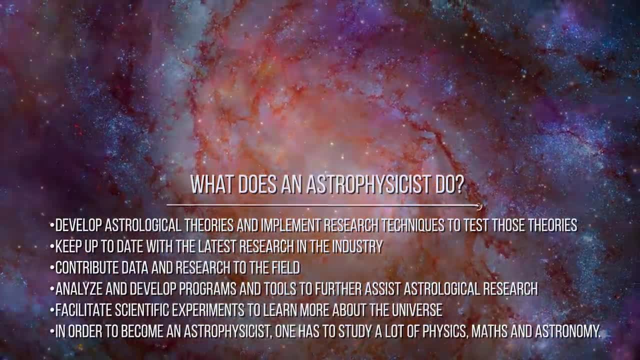 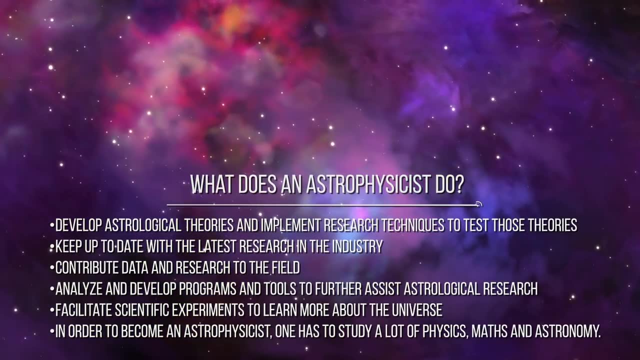 Keep up to date with the latest research in the industry. Contribute data and research to the field. Analyze and develop programs and tools to further assist astrological research. Facilitate scientific experiments to learn more about the universe. In order to become an astrophysicist, one has to study a lot of physics. 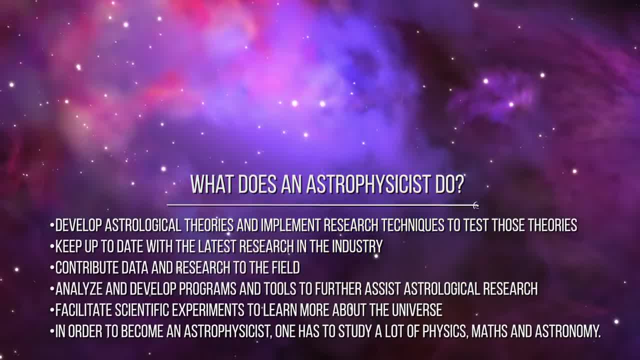 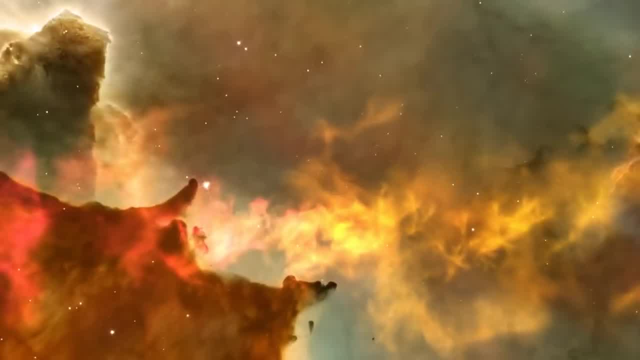 math and astronomy. We could say jokingly that an astrophysicist studies the same physics of a physician, pretty much the same math of a mathematician, plus astronomy stuff. What are the main purposes for a NASA astrophysicist? 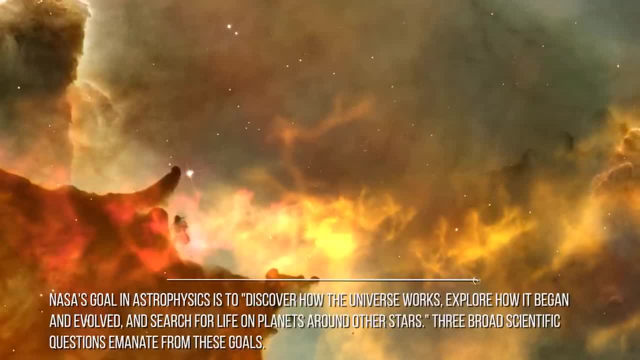 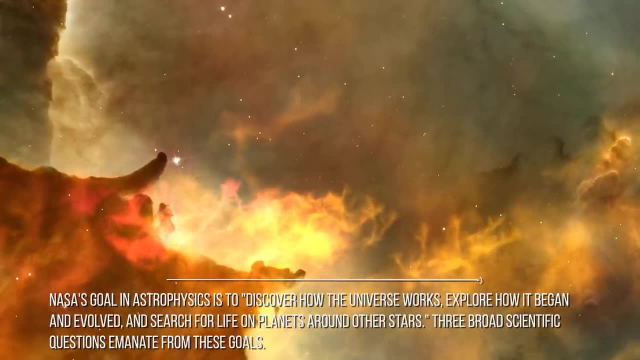 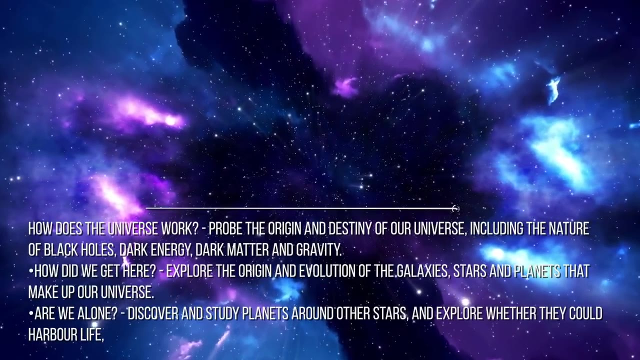 On Nasa's website, we can read: NASA's goal in astrophysics is to discover how the universe works, explore how it began and evolved, and search for life on planets around other stars. Three broad scientific questions emanate from these goals: How does the universe work? 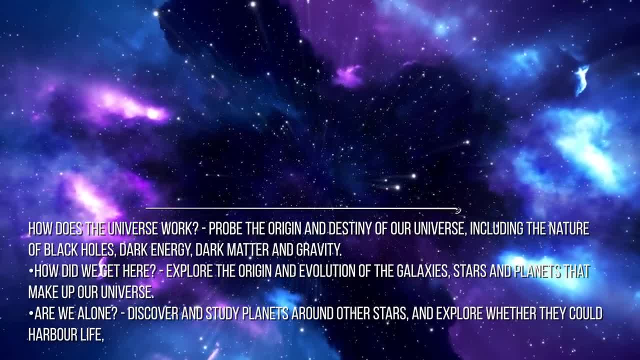